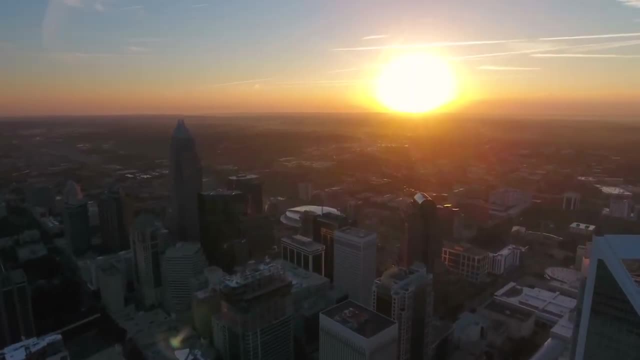 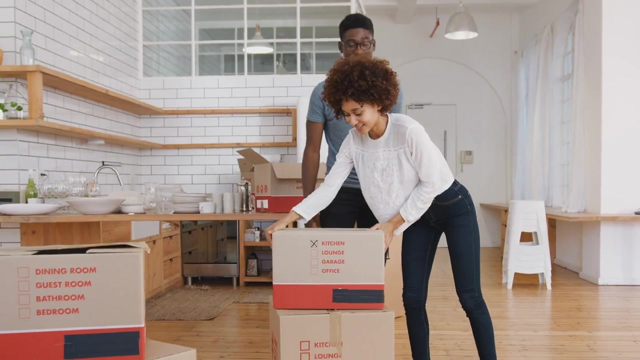 Carolinas to choose, Or maybe you live right here in the Charlotte area, which we are right on the border of North and South Carolina, and you're considering moving from either North Carolina to South Carolina or South Carolina to North Carolina. Today we'll highlight the big differences. 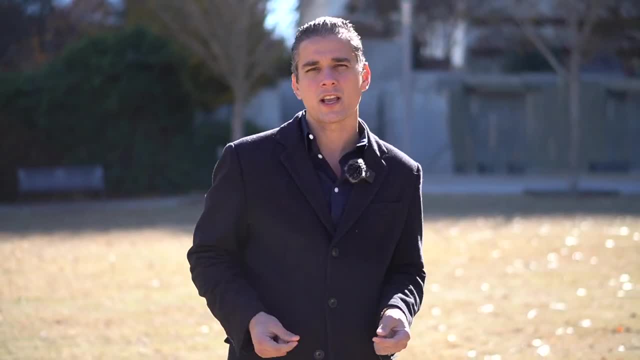 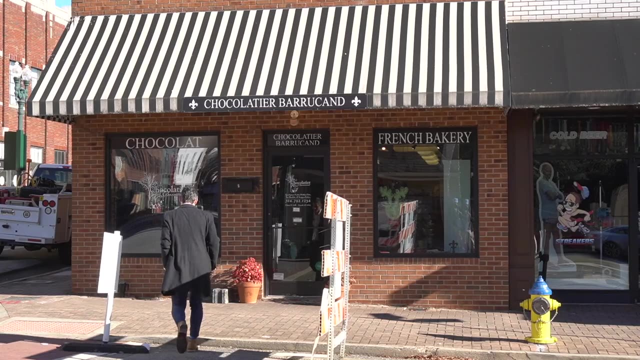 to help you make your decision and make sure you stay tuned till the end, where I give you my opinion on which one's better to live in North Carolina or South Carolina, And I do believe I have a unique perspective because I spent a lot of time living and growing up in both of these respective states. 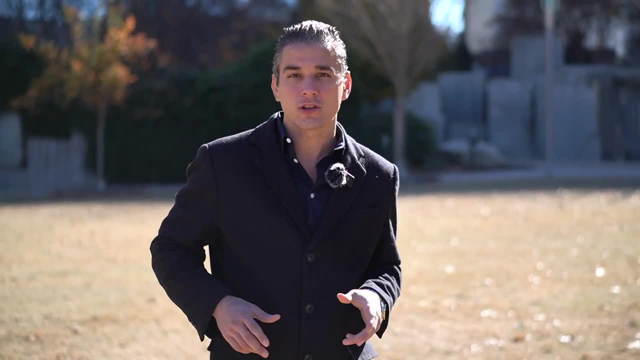 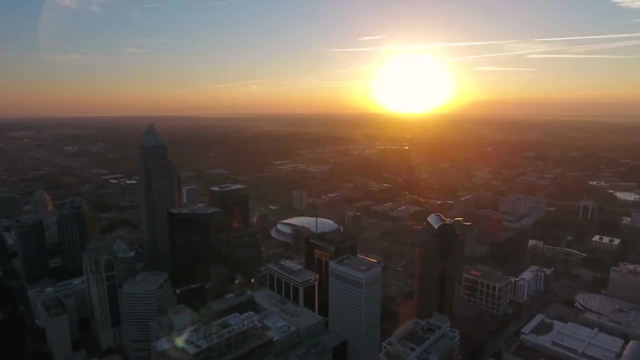 If this is your first time on the channel and you want to know everything there is to know about Charlotte and the surrounding areas, make sure you subscribe to the channel and turn notifications on so you can be the first in the know about the current market here in Charlotte. My name is. 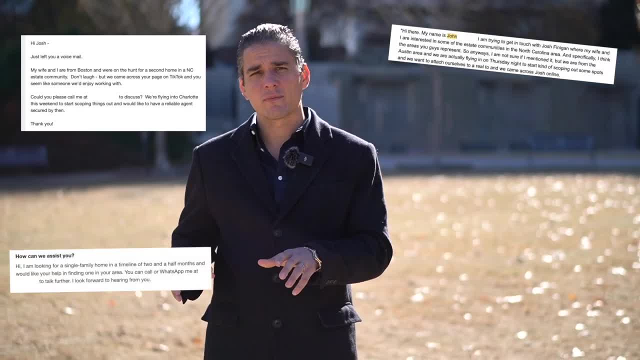 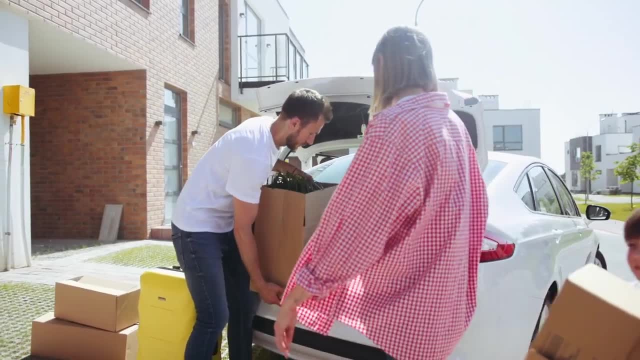 Josh Finnegan, and my team and I get calls, texts and emails from people just like you every single day, looking to move to the Charlotte area, and we absolutely love it. So, whether you're looking to make a move in nine days or 90 days, feel free to shoot us a text, send us an email, give us a call. 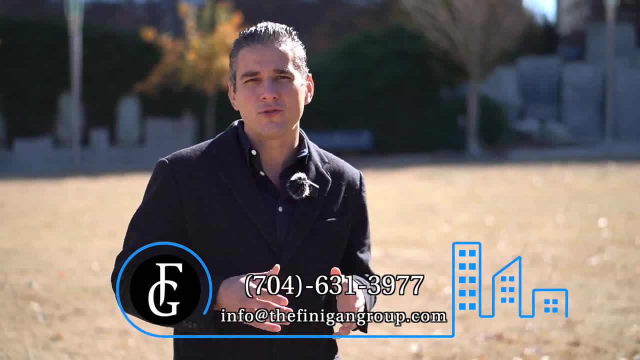 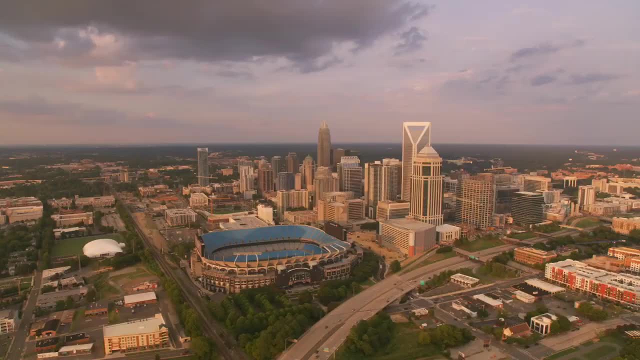 or use the link in the description below To set up a Zoom meeting, which is actually our favorite, so we can put a face to the name. we'd love to help you make an easy transition to the Charlotte area. Now, North and South Carolina share a lot more than just their name. they share a deep, rich history of Southern charm. 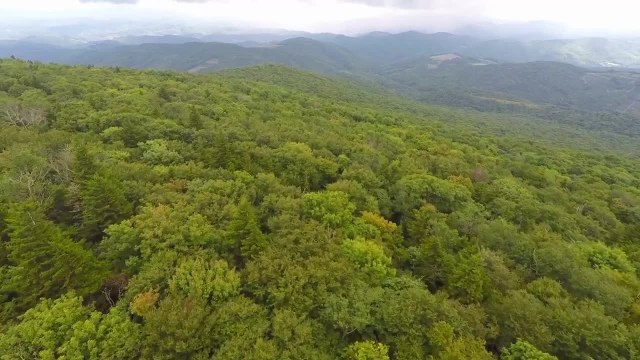 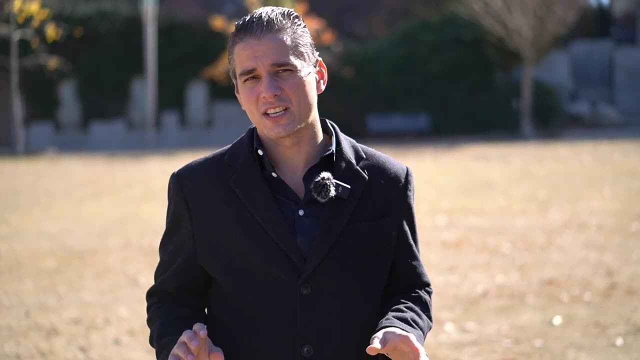 and Southern hospitality. They're also renowned for their beautiful mountain ranges, beautiful beaches, historic cities, tasty barbecue and mild temperatures. But today we're not focusing on the similarities, we're focusing on the differences. So let's go ahead and start off. 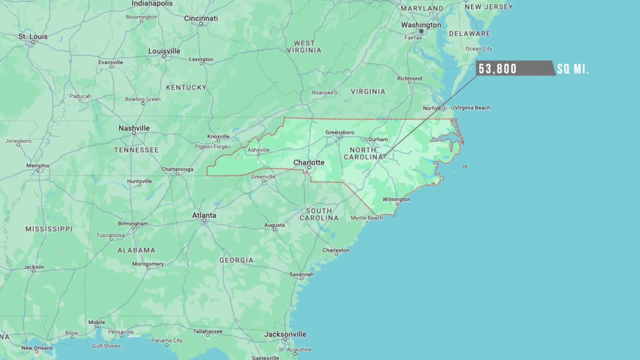 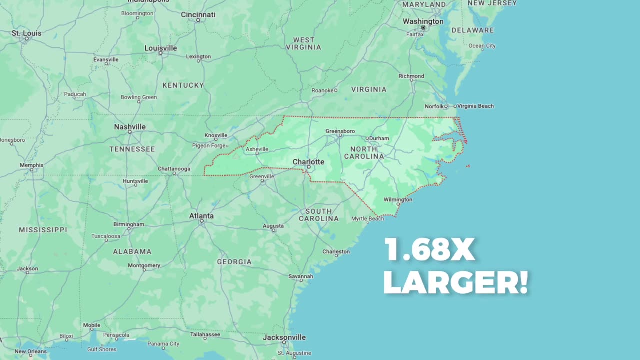 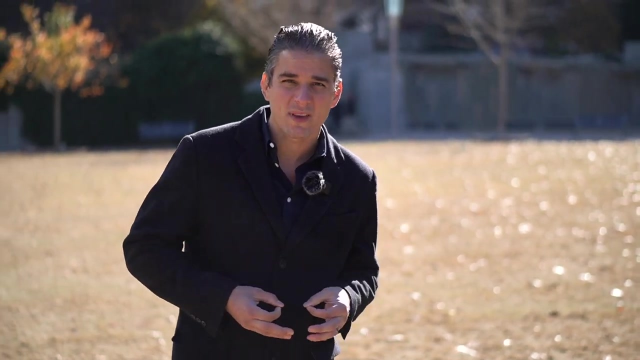 with the facts Now, North Carolina is about 53,800 square miles, where South Carolina is about 32,000 square miles. so North Carolina is about 1.68 times larger than South Carolina. So geographically, North Carolina is much larger, but it also has a lot more people, Based on the 2021 census. North 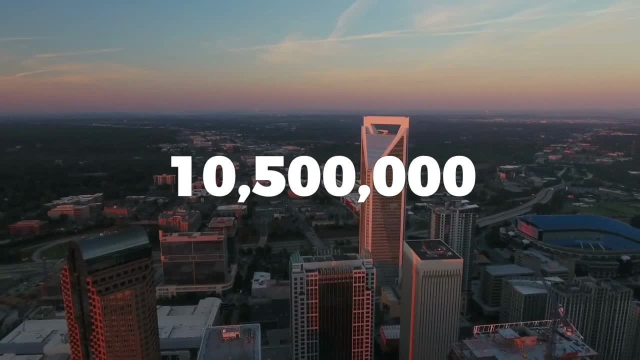 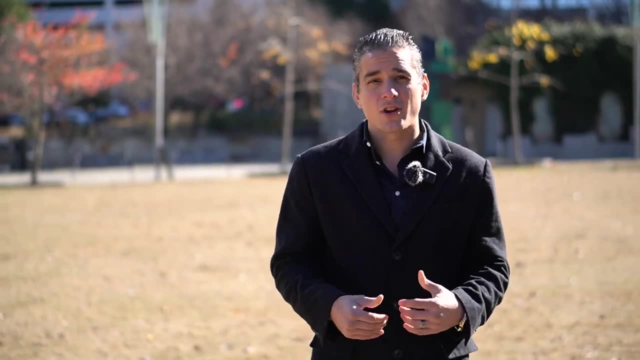 Carolina's population is right around 10.5 million, where South Carolina's population is only about 5.2 million, And North Carolina's population is a little bit lower than South Carolina's population, more dense, so you're going to find a lot more cities in North Carolina than in South Carolina. 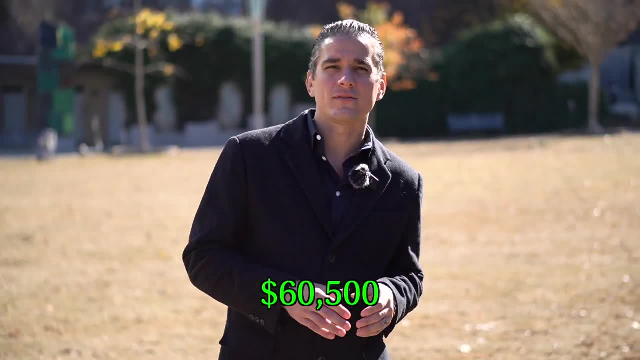 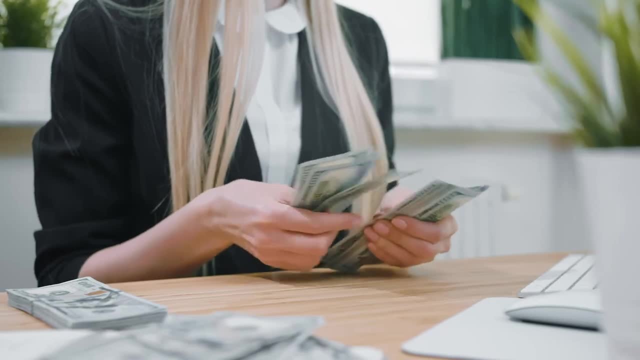 Now North Carolina's median income is sixty thousand five hundred dollars, where South Carolina's median income is just above fifty eight thousand dollars. So the median income of the two states are pretty comparable, but North Carolina does win by just a hair. Now, when we look at the cost of living between North Carolina and South Carolina, they're pretty comparable as well. When looking at the cost of living index, South Carolina is a little bit more favorable, coming in at 89.3, which means the total cost of housing, food, child care, transportation. 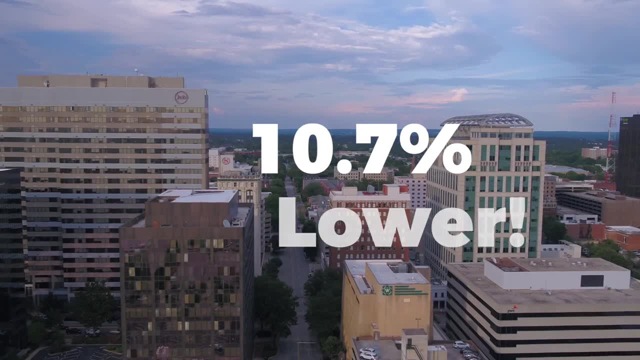 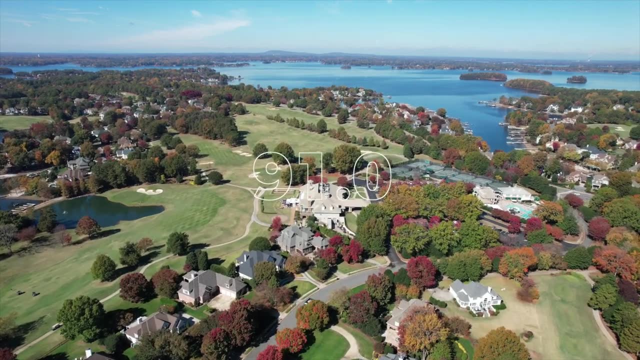 health care taxes and other necessities is about 10.7 percent lower than the United States average cost of living. The cost of living index has North Carolina at 91, so it's a little bit higher than South Carolina but still well below the United States average cost of living. So North Carolina squeaks out a win for median income, but South Carolina takes the cake for cost of living. What about job opportunities? Now? this one's really going to be determined by where you live in these two respective states, but North Carolina is home to major companies like Honeywell. Duke, Lowe's, Epic Games, Bank of America and Truist. South Carolina isn't home to many major companies, but companies like Bosch, Michelin, Boeing, BMW, GM and Volvo all have large plants in the state, So there's definitely a large presence in both respective states for a lot. of these major companies around the world. However, North Carolina's job opportunities are going to be determined by where you live in these two respective states. But North Carolina's home takes the cake for more companies and more headquarters. But North Carolina and South Carolina both have very strong job markets, particularly in industries like technology. healthcare and education. But North Carolina does have a larger overall economy, so you're probably going to find more job opportunities in North Carolina versus South Carolina. Plus, North Carolina has a lot more major cities, like Charlotte, like Raleigh, Asheville, Durham and Wilmington, Where South Carolina has fewer major cities, so it's probably better for tourism. 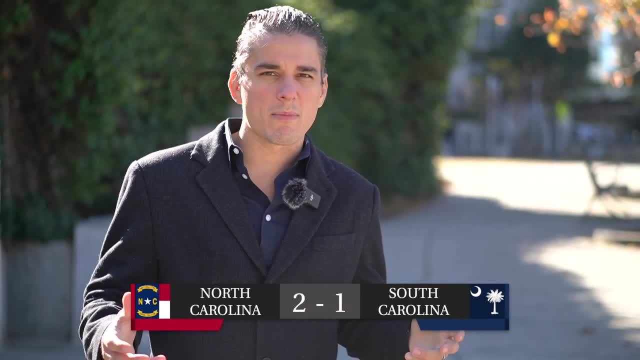 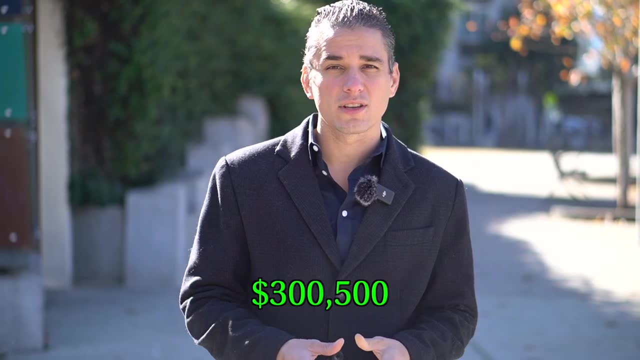 manufacturing and manufacturing. So we have to give North Carolina the win for job opportunities. So let's look at the average sales price In South Carolina. over the last year, the average sales price has been $300,500, while in North Carolina it was slightly higher at $329,500. So, unless you're looking to pay more for a house, South Carolina wins this one. But I will say the average sales price in South Carolina rose 19.2% over the last year, while North Carolina only rose by 15.7%. So both North Carolina and South Carolina have higher sales prices than South Carolina. So both of these areas are in high demand. We have a lot of people moving to the Carolinas- either North or South Carolina- But South Carolina did have a little bit more appreciation over the last year. Now these average prices will vary very greatly between where you're living within these states. Right, the bigger cities you're going to have a higher price point than the more rural areas, And North Carolina has more major cities, so that's really going to affect the average sales price in North Carolina versus South Carolina. Which brings us to the next point. If you are looking for more, 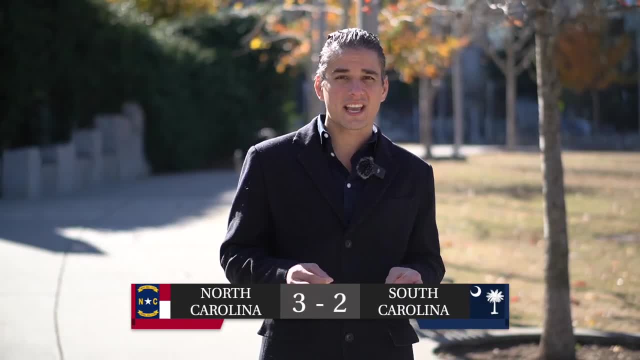 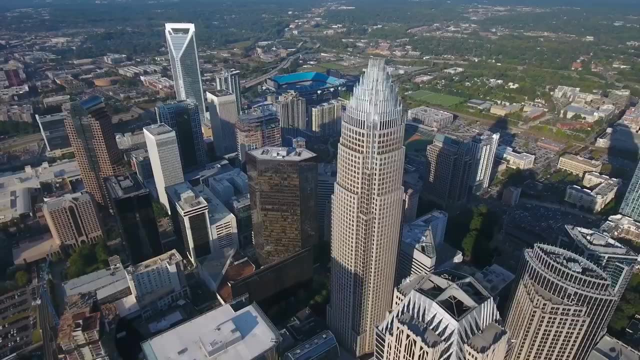 major cities to choose from, North Carolina definitely takes the cake. You're going to find a lot more major cities that have a higher population and a more densely populated area than South Carolina. Like we mentioned earlier, in North Carolina you can find many major cities like: Charlotte, Raleigh, Durham, Greensboro and Asheville, just to name a few. South Carolina does have major cities, but they are few and far in between. There's a lot more rural area in South Carolina. You will find major cities like Columbia and Charleston. 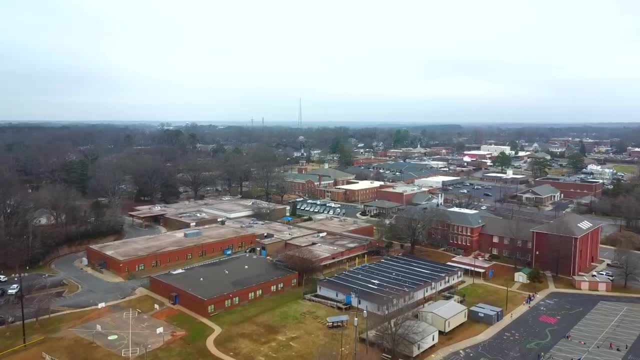 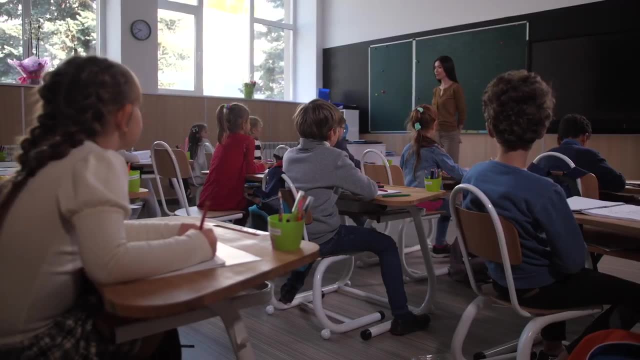 But in between them there's going to be a lot more rural, smaller towns. But don't be fooled, because North Carolina does have some super cool rural towns you've never heard of as well. So let's take a look at the education and, guys, I will tell you, education is one of the buyers top. 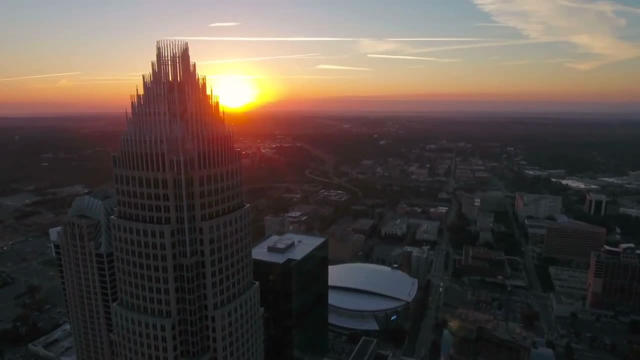 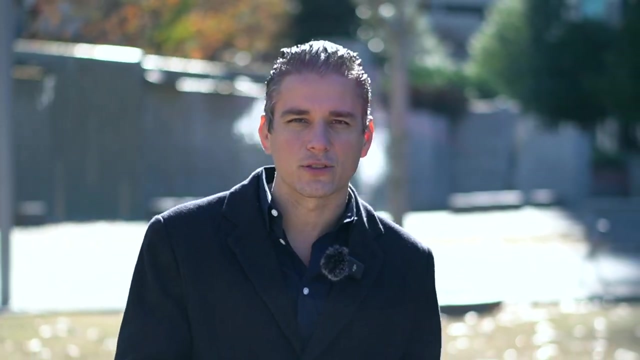 three questions they have. when moving to the Charlotte area. They'll ask: Josh, how are the schools, Where are the best school districts And where should we be looking to get in the best schools? When it comes to public education, both North and South Carolina are one of the 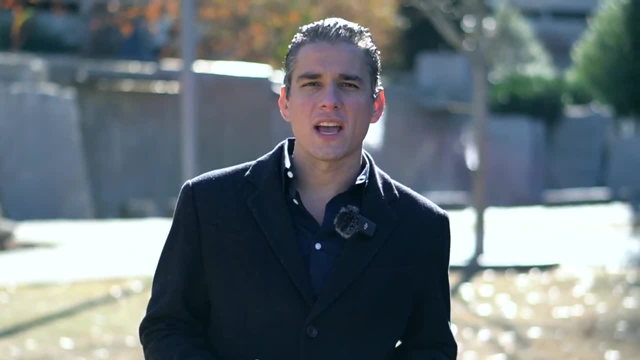 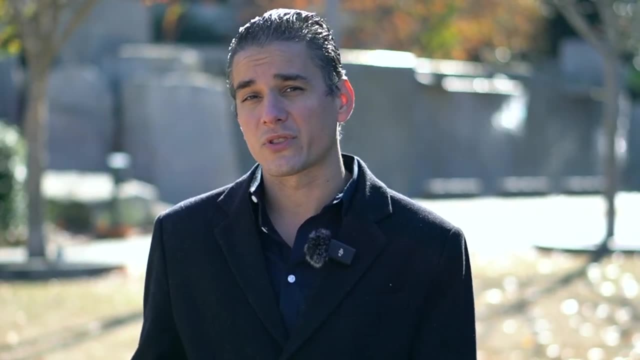 best places to look. They are well known for their strong school systems. Now, North Carolina has a higher population and is more population dense than South Carolina, So you're going to find more schools and more students in North Carolina versus South Carolina. Now North Carolina does rank. 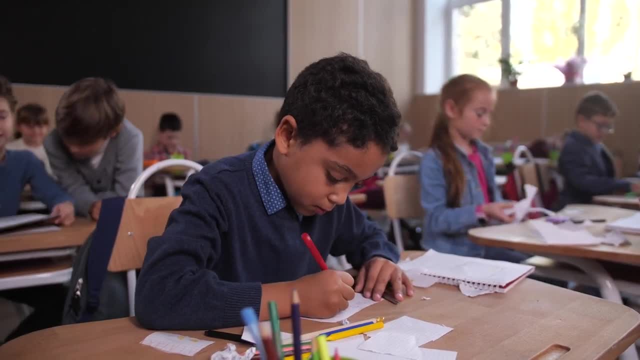 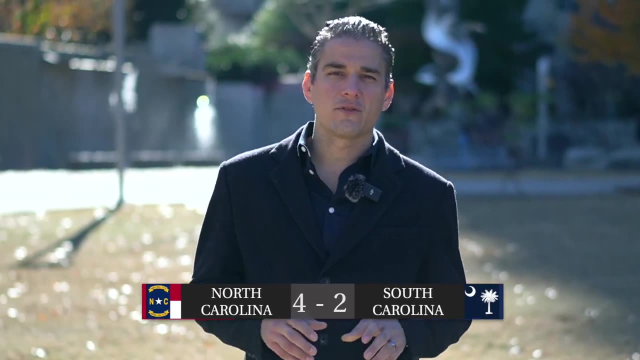 slightly higher than South Carolina when it comes to looking at the education system overall, Because it does have slightly higher test scores and graduation rates. Because of this, I do have to give North Carolina the win on education, But I do personally think it is very location. 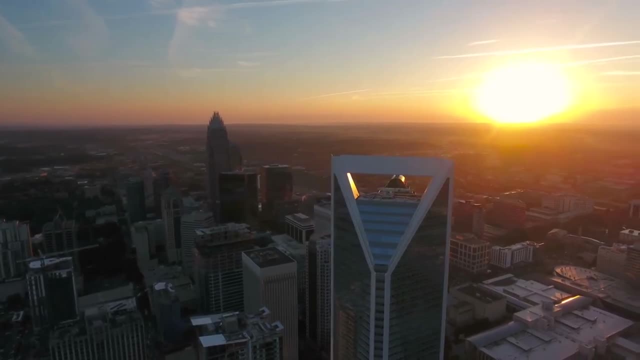 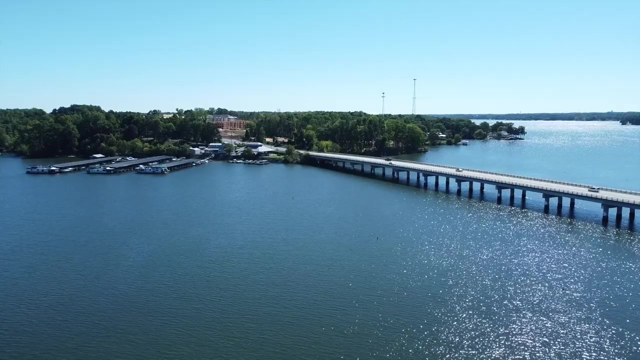 specific. So we're here in the Charlotte area, So I service both North and South Carolina. A lot of our clients actually move from Charlotte to South Carolina just across the border, in towns like Lake Wylie or Fort Mill, specifically because of the better schools. One last point on the school. 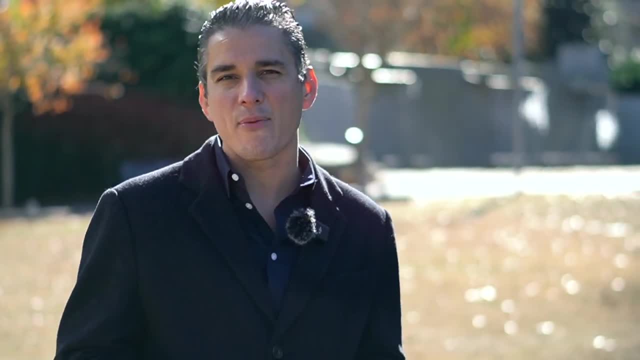 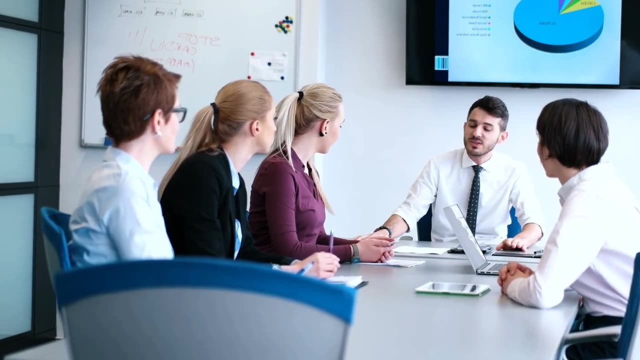 systems here in North and South Carolina is. they do both operate in very similar ways. They both operate on districts run by locally elected superintendents and school boards. So what about higher education? What about higher education? What about higher education? What about higher? 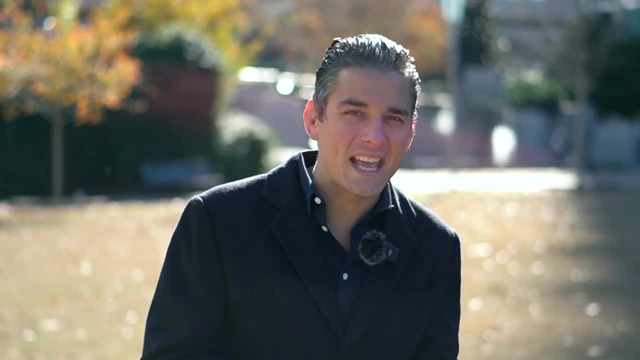 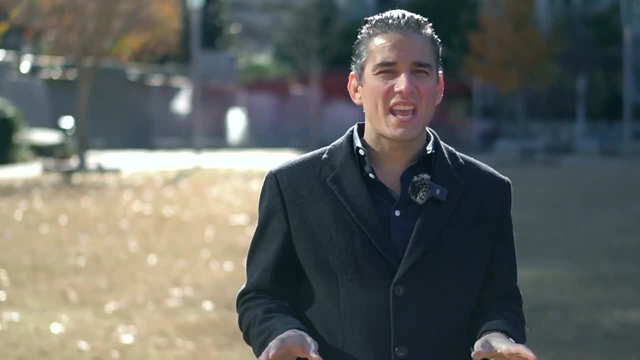 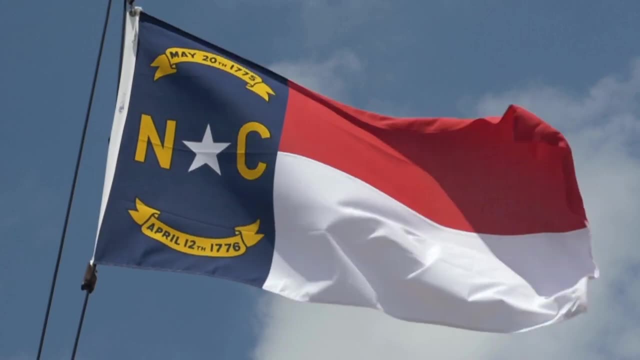 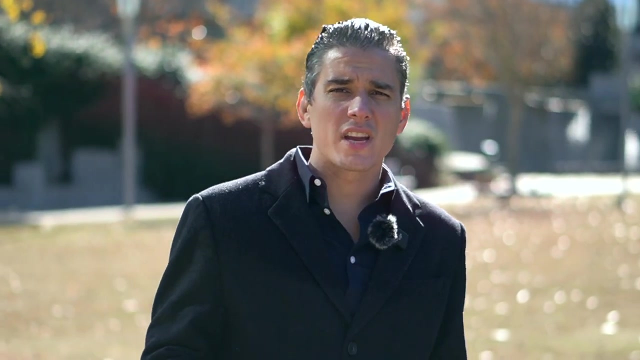 attractively priced than out-of-state tuition. Both states have some excellent choices when it comes to higher education. North Carolina is home to some of the best colleges and universities like Duke, UNC, Chapel Hill and NC State. North Carolina does also have a lot of great options for some small. 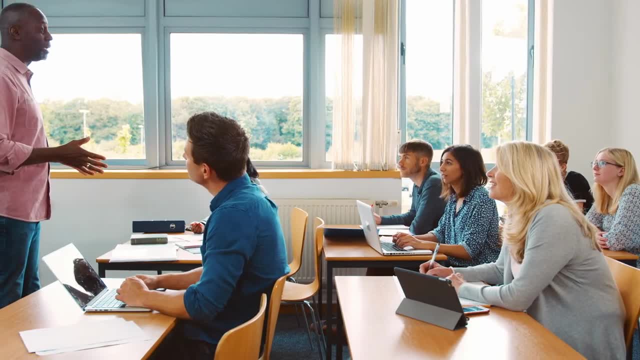 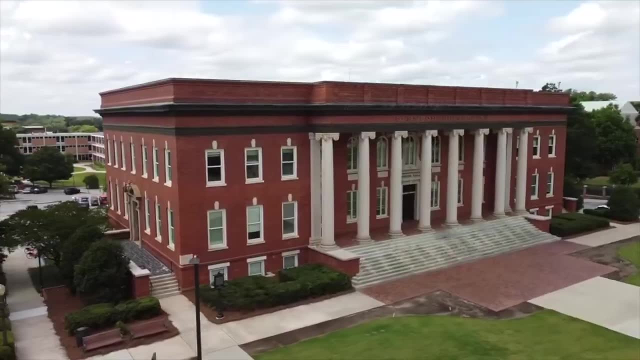 private liberal arts colleges, mid-sized colleges and large research facilities. Now, South Carolina does have some awesome colleges and universities as well. Most known is USC and Clemson. They're not as well known as the North Carolina schools, but they are fantastic in their own right. Now I went. 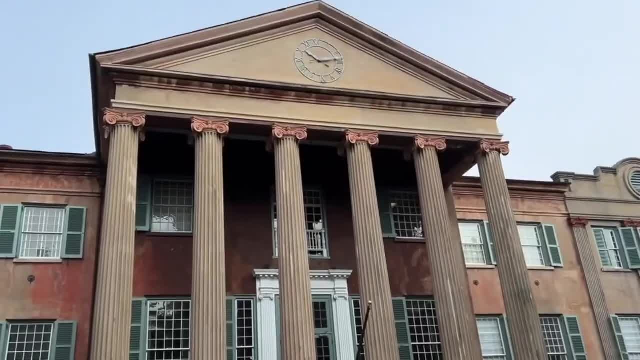 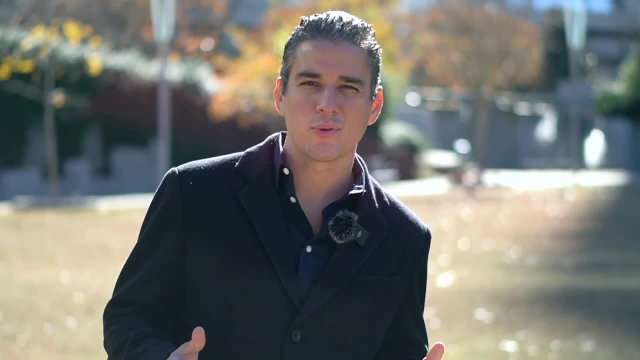 to the College of Charleston. I love that school. A little bit smaller, but it has a great education potential. So both these states really have some fantastic options for higher education. They rank high across the board in academics and also in sports as well. So NC does have more universities. 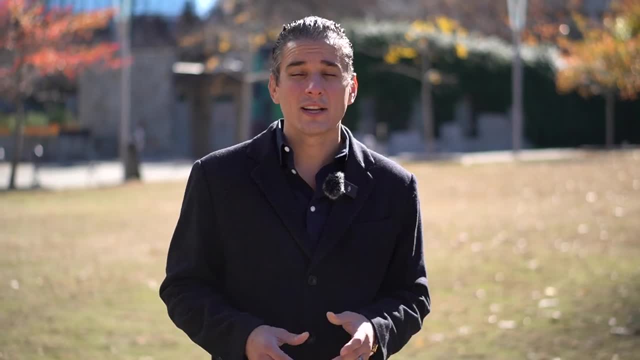 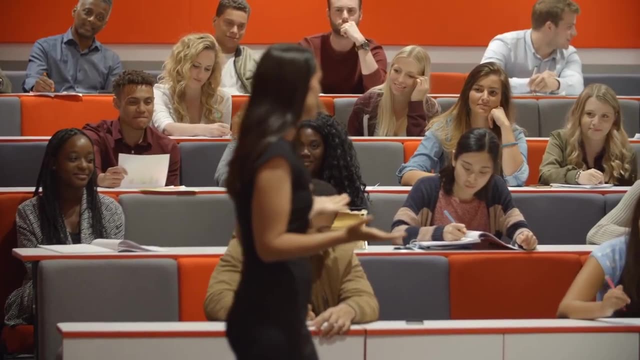 and colleges to choose from, and they're a little bit more diverse than the rest of the state, So they're a little bit more well-known. So I do reluctantly have to give North Carolina the win on higher education, but in my opinion it really boils down to what you were looking for in a 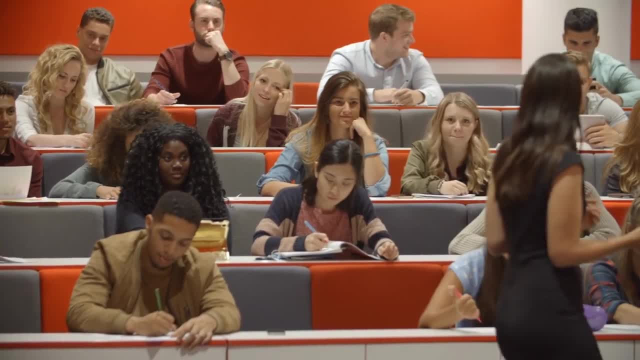 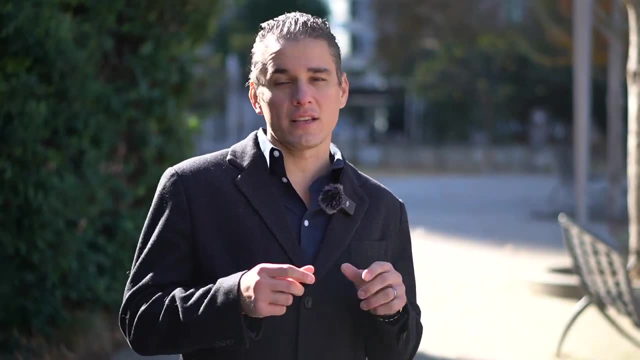 college, right? What are you looking to major in? What kind of lifestyle do you want? So how about the climate? Now? North and South Carolina's climate is going to be pretty similar Now. South Carolina is obviously south, so it's going to be a little bit warmer, while North Carolina is going to be a little bit cooler Now both Carolinas do experience hurricanes, which is something you should really be aware of, So the weather patterns really vary more east to west than they do north to south, meaning it's warmer at the coast and cooler in the mountains of both states. Now I absolutely hate cold weather. And again, South Carolina is slightly warmer than North Carolina, So I do have to give South Carolina the win on this one. So let's go ahead and talk a little bit about the great outdoors and topography. Well, if you're looking for the mountain terrain, then North 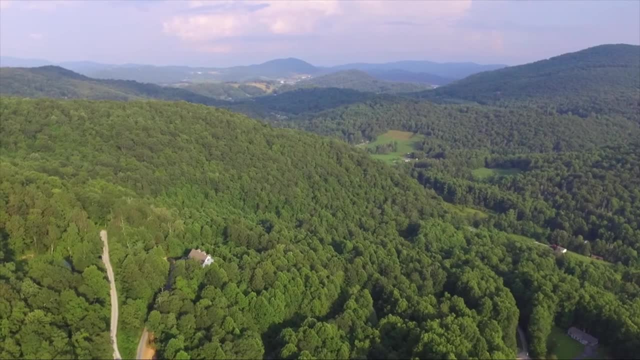 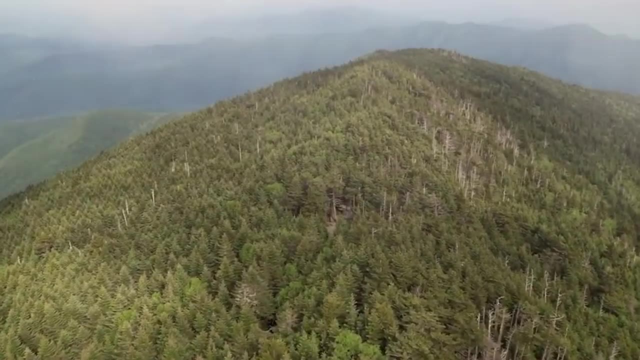 Carolina definitely takes the cake on this one, And that's because about one fourth of North Carolina has mountain ranges, From the foothills all the way up to Mount Mitchell, which is the highest point on the east coast. you're going to find a lot of mountain ranges right here in North Carolina. 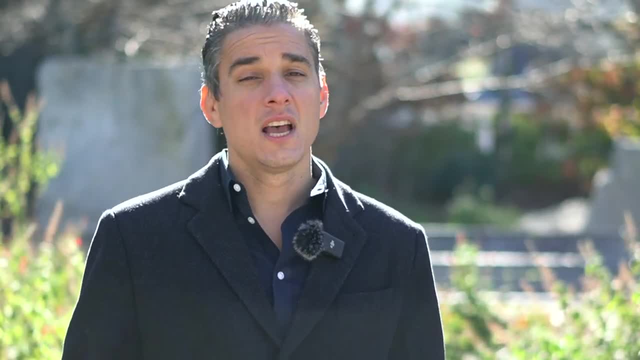 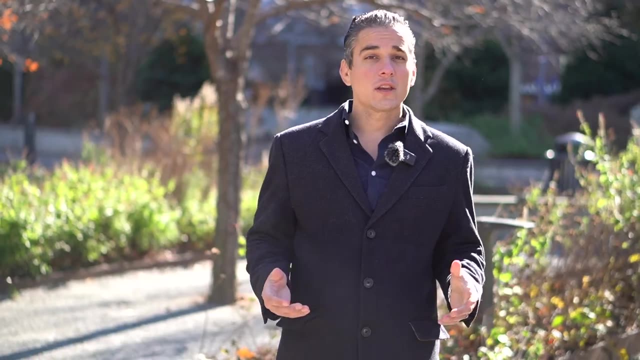 North Carolina also has some super cool mountain towns that either is great to live in or for a quick day trip. You can visit Boone, Asheville and Blowing Rug. If you are looking for mountain activities- whether it be whitewater, rafting, skiing, hiking, ziplining- you're going to find. most of those activities in North Carolina over South Carolina. So if you're looking for a little bit of that, then North Carolina is definitely the winner. Now South Carolina again does have mountain ranges, but they're up to the northwest part of the state and there's not much activities. 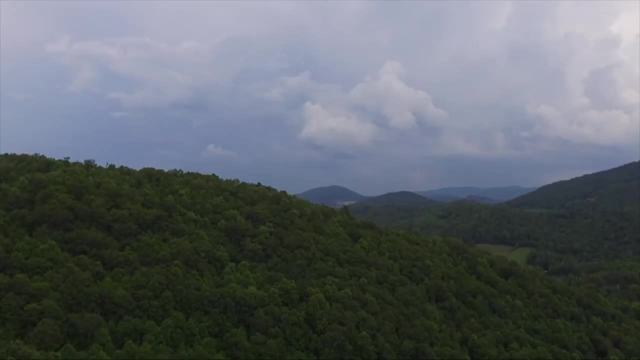 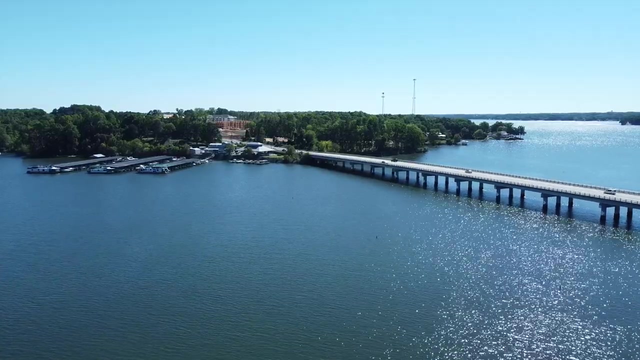 you could do there. So if mountains are important to you, then North Carolina is definitely the clear winner here. But let's go ahead and talk about the lakes guys. And again, North Carolina does win this one, because you're going to find a lot more lakes in North Carolina than in South Carolina. South Carolina has 12 major lakes, where North Carolina has 59 major lakes. North Carolina is, which is the largest man-made lake on the east coast And actually where we live and work here in the Charlotte area. we actually have three lakes: Lake Norman Mountain, Island Lake and 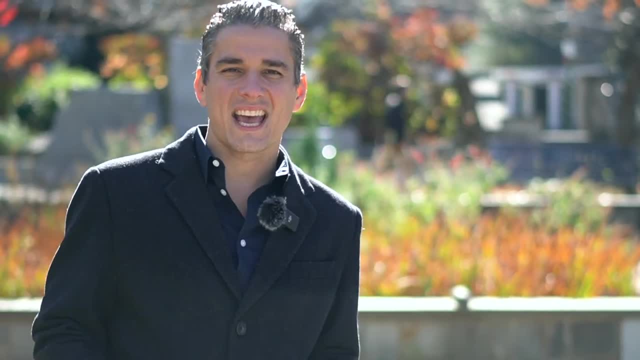 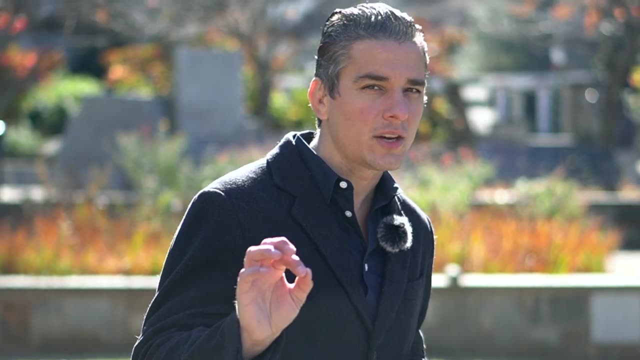 Lake Wiley, which gives us Charlotte residents fantastic access to wonderful lake life. But if you want to know a little bit more about lake living here in the Charlotte area in particular, we shot a whole video going through Lake Norman Mountain Island Lake and Lake Wiley. I'll put. 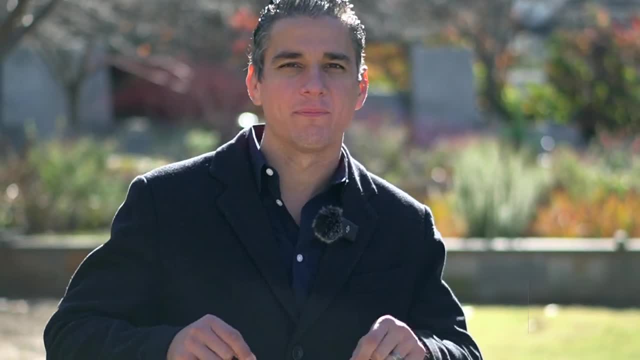 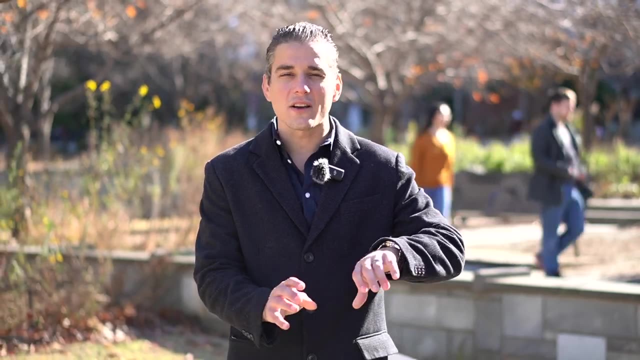 the link to that video up here in the corner and also in the description below. Now I will say North and South Carolina. both do share Lake Wiley, but besides Lake Wiley, South Carolina does have some fantastic lakes all their own. You have Lake Marion and Lake. 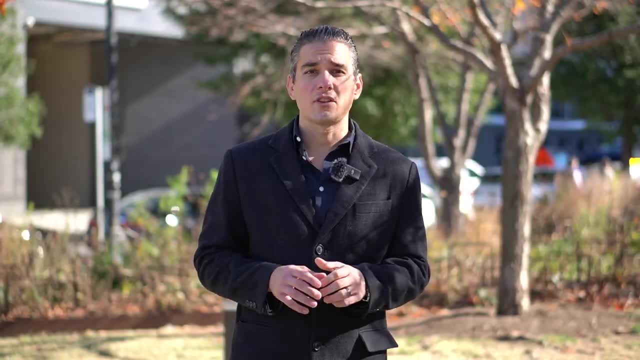 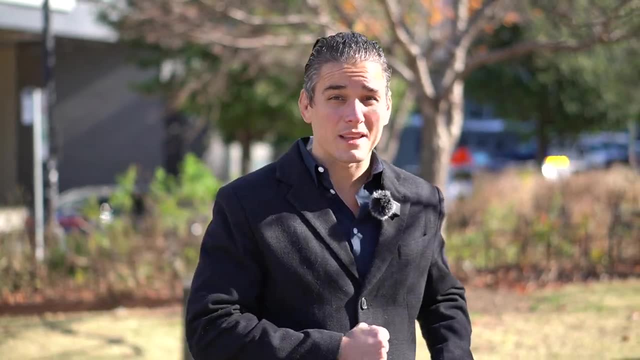 Moultrie, which you can find between Charleston and Columbia. You have the Clark Hills Lake, which is actually on the border of South Carolina and Georgia, which is the second largest lake on this side of the Mississippi- Sorry, guys, I just always wanted to say that- And you have Lake Murray. 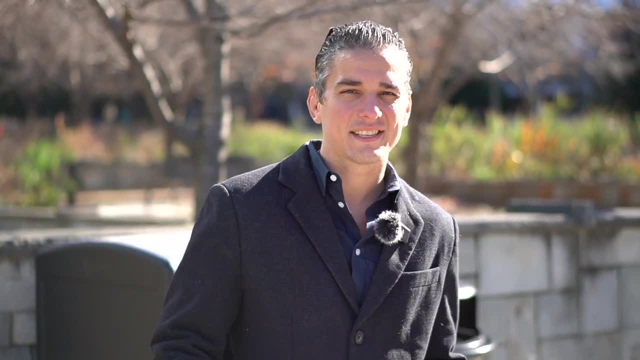 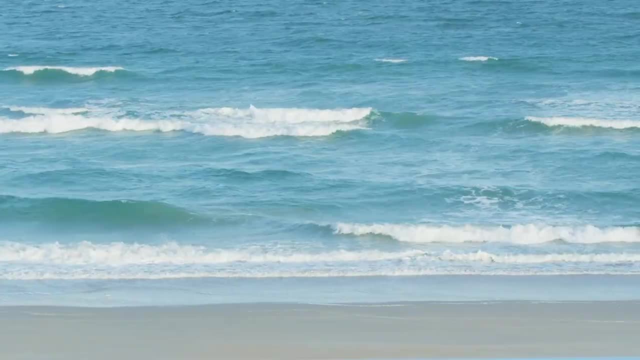 and Lake Wiley. So North and South Carolina both give you fantastic options for great lake living, but I do have to say North Carolina does take the cake because they have a lot more. So let's go ahead and talk about some beautiful beaches, which hopefully it'll warm me up a little. 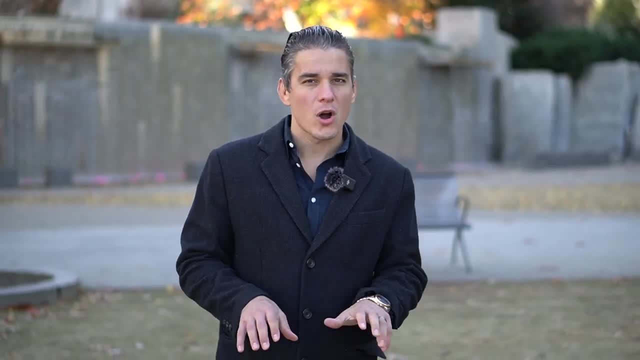 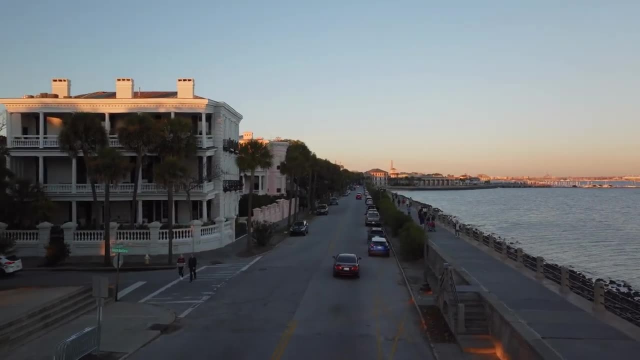 bit on this cold day to think about. But this one's definitely going to be a really hard one, because both North and South Carolina has some fantastic options when it comes to beach towns. Now I may be a little bit jaded because again I did go to College of Charleston. I love Charleston. 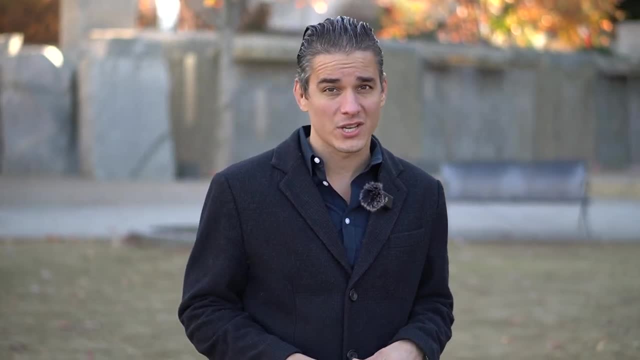 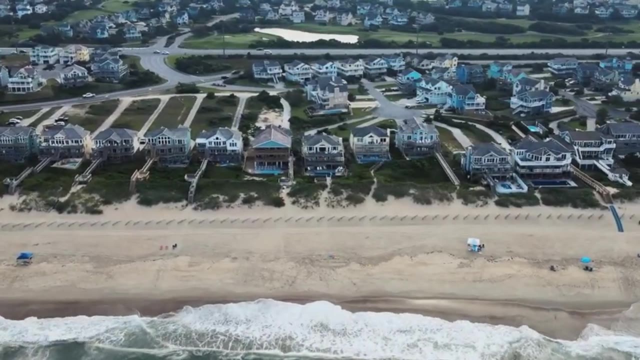 My wife and I visit there. We still own property in Charleston as well, But North Carolina does have one of the largest coastlines on the East Coast. Now in North Carolina you do have the Outer Banks, which is very well known. Now, I personally haven't ever been to the Outer Banks because it's about 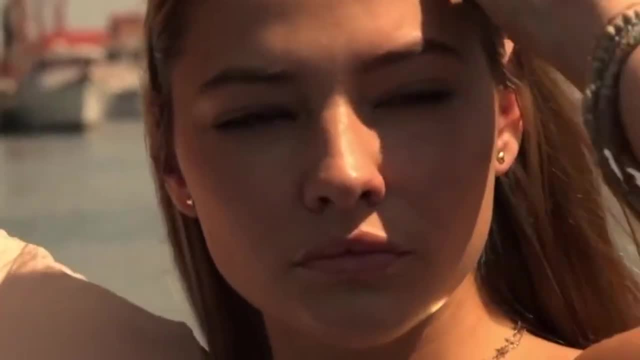 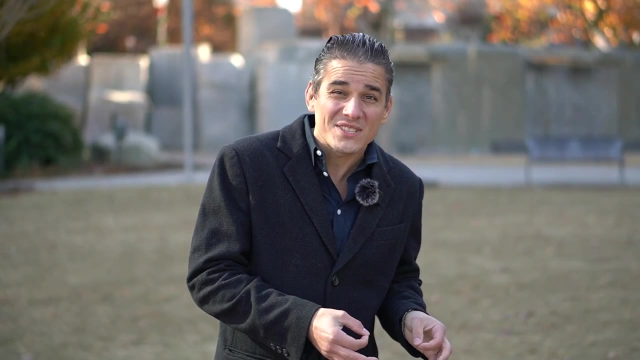 six and a half seven hours away from Charlotte, And many people know the Outer Banks because of the super popular TV show Outer Banks. But fun fact, Outer Banks was actually filmed in Charleston, So that is a win for Charleston. But you also have Wilmington. 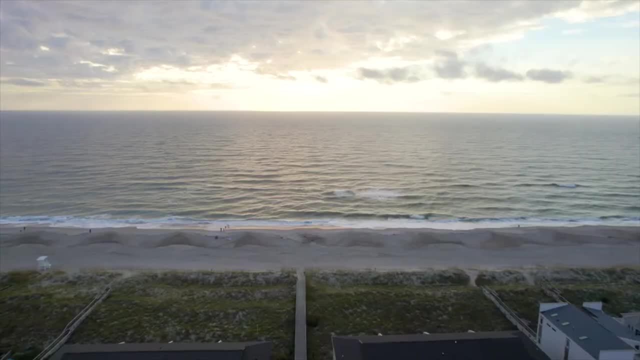 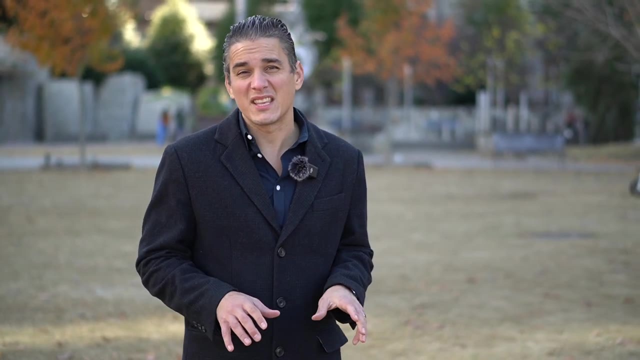 a lot of the coastal cities. on the coast It's actually like a mini Charleston. They also have Carolina Beach. You have Oak Island. A lot of choices in North Carolina. But one thing I've personally noticed: in my opinion it's a little bit harder to get to the coastal cities in North Carolina than it is in South Carolina. In North Carolina there's a lot more smaller windy roads to get to these coastal cities, which can take you a little bit longer than in South Carolina, where you do tend to have some larger highways that take you directly to the city. Now, South Carolina has some fantastic beach towns. 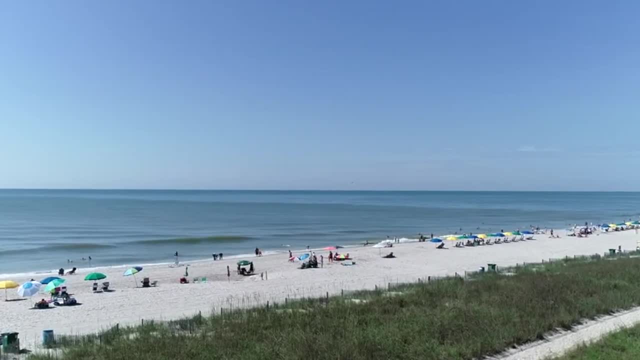 Now South Carolina has some fantastic beach towns. It's a great place to come to And if you're willing to spend a little bit of your time here, it's probably worth it. Now I've been to the the city. now south carolina has some fantastic beach towns to visit. you have myrtle beach you. have charleston and you also have hilton head, another super cool town to visit. you'll also find more hotels available in south carolina, especially in that myrtle beach area, so in beaches overall, while both states have some gorgeous beaches, south carolina does take the cake, in my opinion. so how about history? which state has more historic histories? now, both states are deeply entrenched in united states history in general, but you're going to find more historic towns in north carolina, frankly, because it's larger, there's more cities, but south carolina definitely wins, in my opinion, for the best historic city: charleston, south carolina. charleston has some exquisite historic plantations and homes and you will absolutely love going downtown historic charleston, seeing all the rich history and beautiful churches everywhere and in north carolina. you can visit some fantastic historic towns in north carolina and you'll find some. historic towns as well, like brevard, ashville or wilmington, and south carolina has some other great options other than charleston. you have bluffton and butteford. so north carolina does win for having more historic towns, but south carolina wins for having the best historic town. so how about something that everyone loves to talk about, especially in april every single year, and that is the tax burden? now, generally, you're going to find that north carolina has a higher tax burden than south carolina. when you take a look at the overall taxes, you 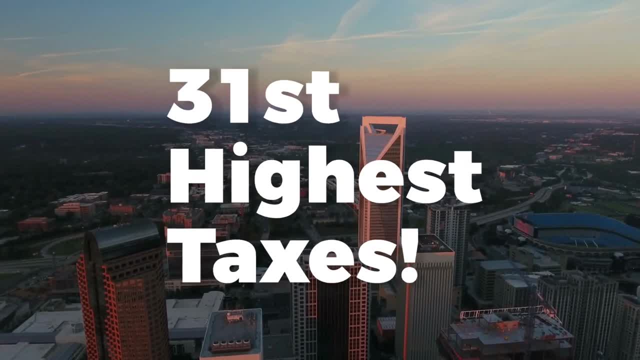 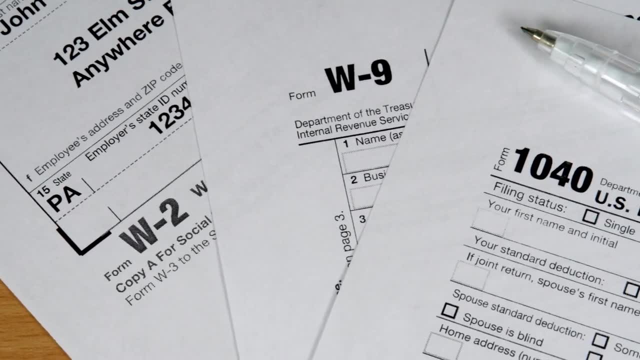 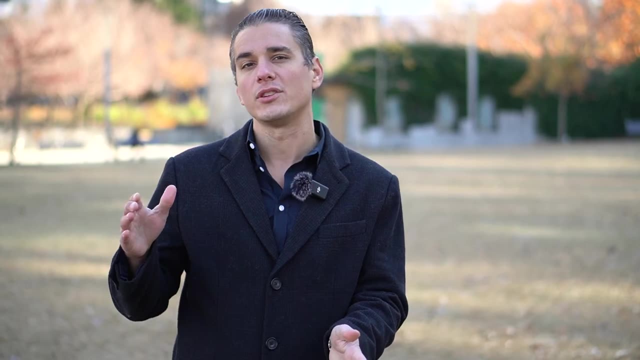 pay. north carolina ranks as the 31st highest taxes in the united states, while south carolina ranks as the 40th in highest taxes in the united states. now, both of them do have income taxes. north carolina has a graduated income tax rate ranging from 5.25 up to 7.75. south carolina has a flat income tax of seven percent. neither state has social security tax, which is a nice benefit. north carolina has a five percent, while south carolina has a state sales tax of six percent. now, north carolina does tend to have higher property taxes as well, but north carolina also has only one property tax. rate. so whether you own a property as a primary resident or an investment property, it's going to be the same rate here in north carolina, where south carolina generally has lower property taxes. but that's for primary occupant owners. south carolina has two different tax rates you have. 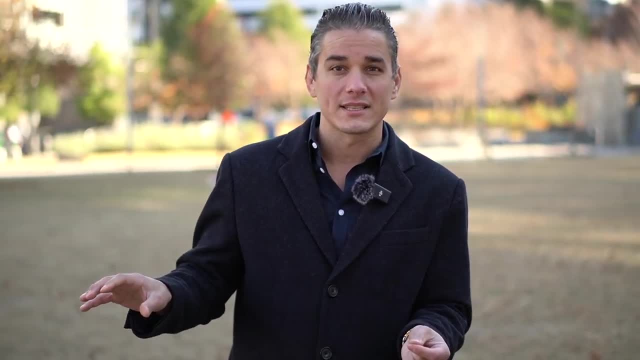 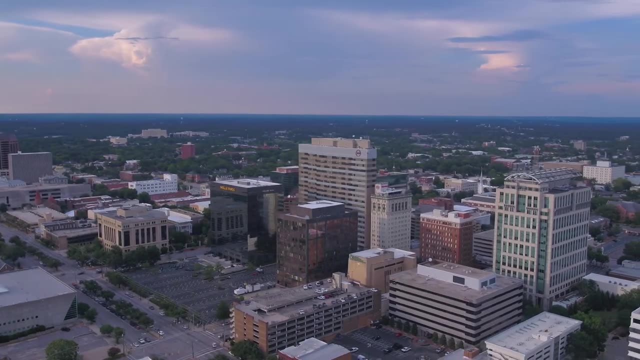 a primary residence, and then you have a state sales tax, and then you have a state sales tax and then you have a secondary residence. now the secondary residence is taxed at a higher rate, and it could be three times as high as if it was your primary occupant. so if you are looking for 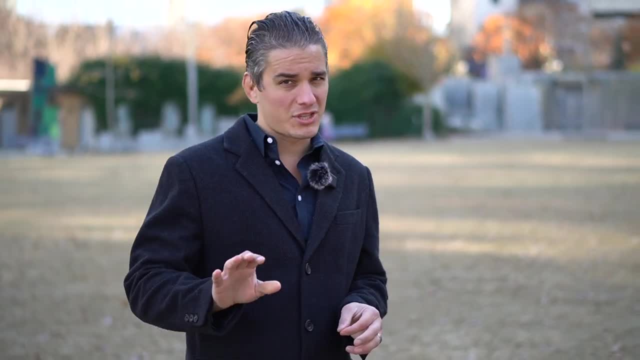 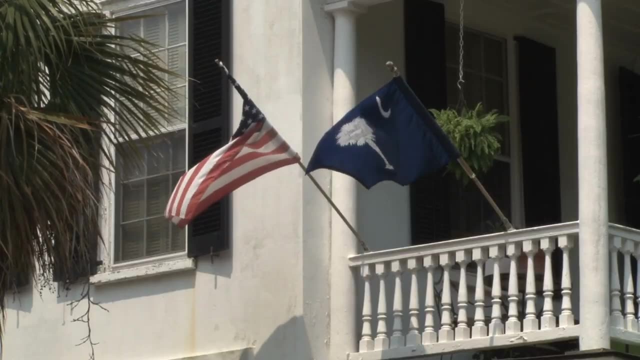 investment property in south carolina. make sure you double check the property taxes before actually purchasing the property, because you could be set up for a rude awakening also for those of you who are purchasing a primary residence in south carolina. you have to apply for your primary. 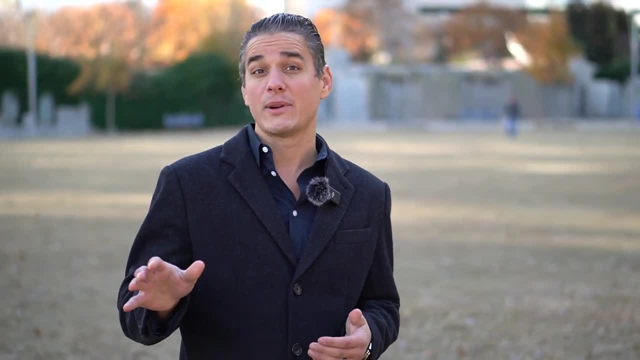 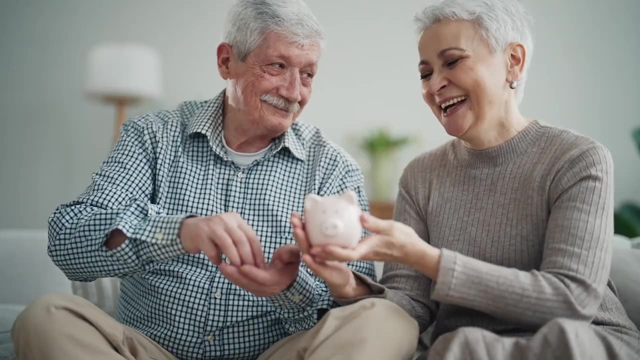 residence tax rate. if you don't, they're going to go ahead and tax you at the higher rate, which could be quite a big surprise when it comes to paying your mortgage. so if you are retired, retirement income tax is more favorable in south carolina, now neither north or south. 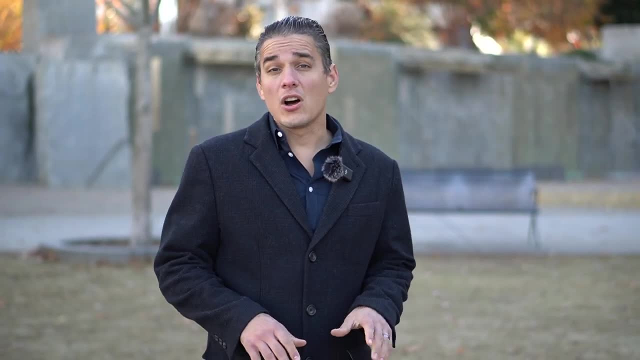 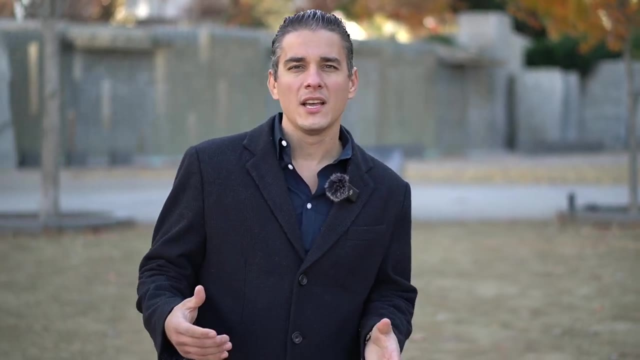 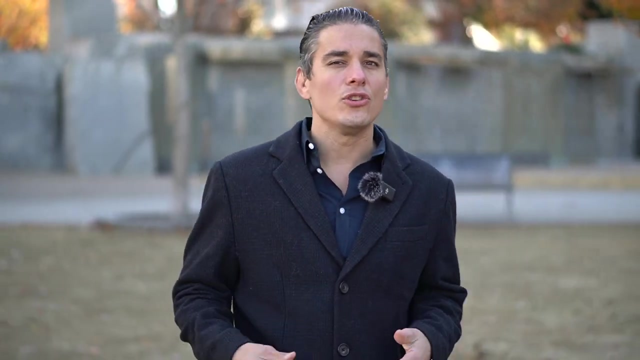 carolina have estate or inheritance tax, so taxes are very subjective. i always recommend talking to your tax advisor if you are considering either north or south carolina and they'll be able to help you with you and your particular goals and situation. but if you look at a grand scheme usually 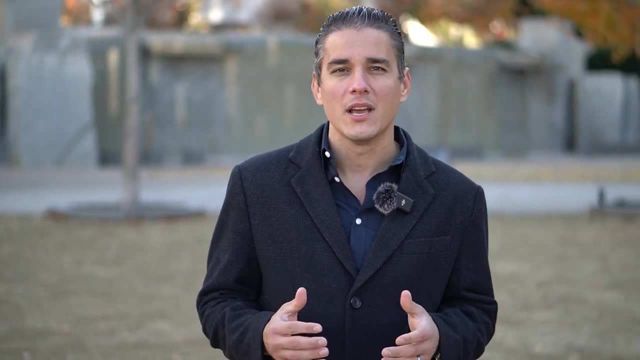 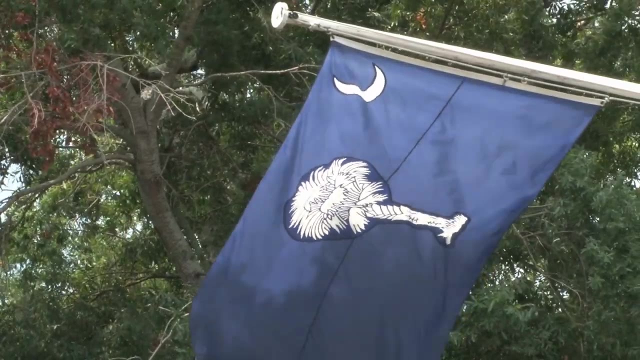 south carolina is more favorable when it comes to a tax burden, which is why a lot of people in our area work in charlotte and actually commute home every day, just across the border and live in south carolina, and because of this, we're going to give south carolina the win for the tax burden. 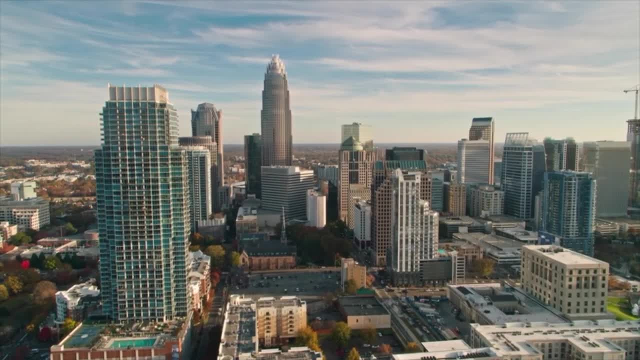 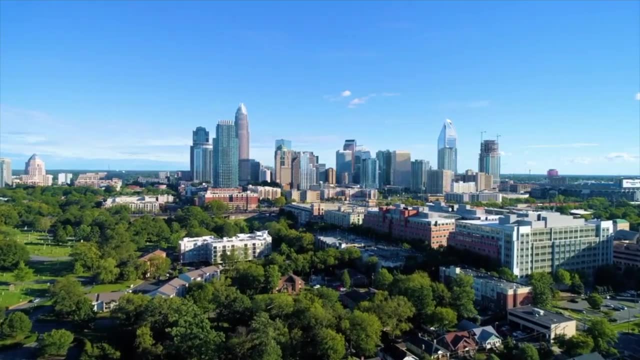 and so that's really the biggest differences you're going to find between north and south carolina, and in my opinion they do have a lot more in common than they do have differences. but i did tell you, if you stayed till the end, i would give you my personal preference. i'm gonna give you my personal preference on either north or south carolina. i grew up in the greater charlotte area in a town called clover, south carolina, just across the border of south carolina, and i currently live in charlotte, actually on mountain island lake, so i own. property in both north and south carolina. i've lived in north and south carolina so i know a lot about both these states respectively, and i really do think both these states are great. if you are looking for a lower cost of living, lower home prices and great schools, south carolina may be a.